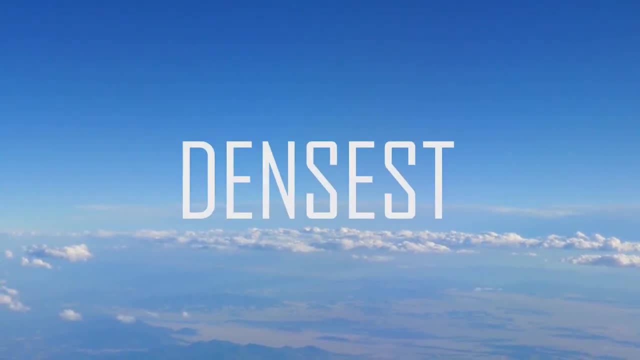 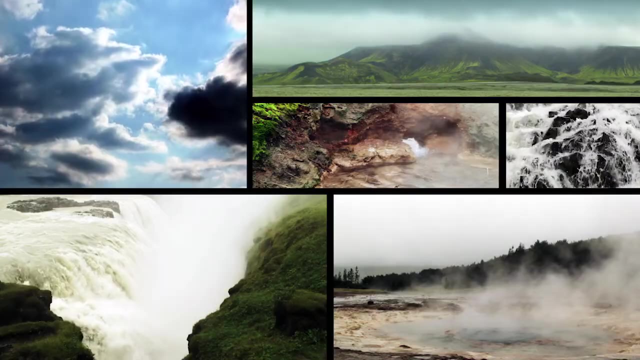 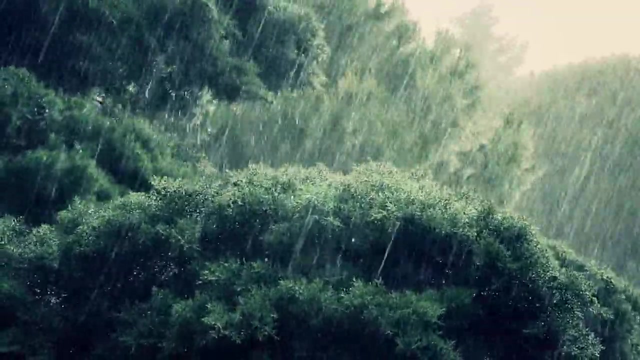 miles in the air. This layer is the densest, meaning it has more particles and heavier gases than the other levels. The majority of Earth's weather occurs within the troposphere. This layer is also the warmest at the bottom, as it is closer to the heat that the Earth is absorbing from the 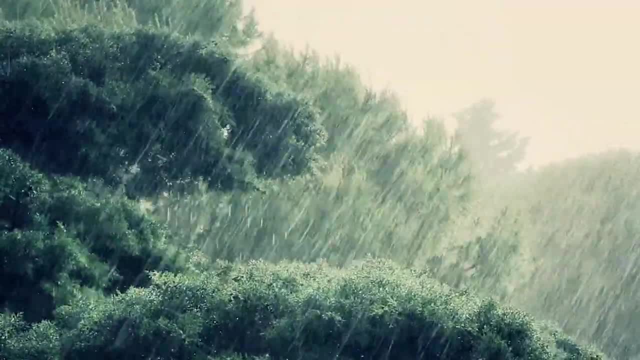 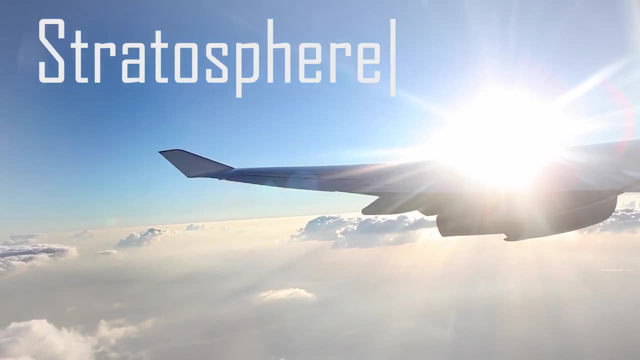 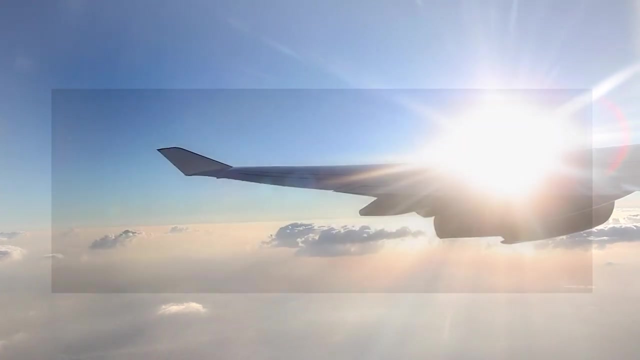 sun. As you go farther up into the troposphere, the temperature drops. The next layer that begins at the top of the troposphere is the stratosphere. The stratosphere stretches for about 30 miles outward into space. This layer is the maximum height at which jets can fly The stratosphere. 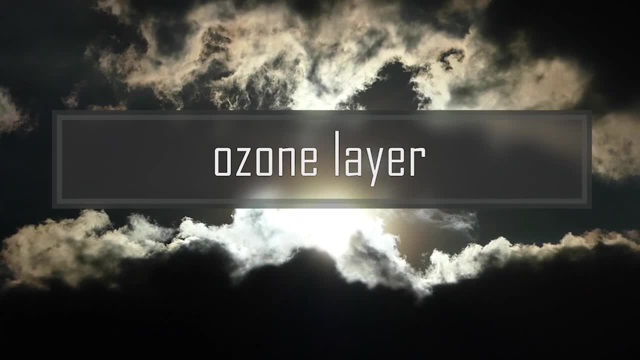 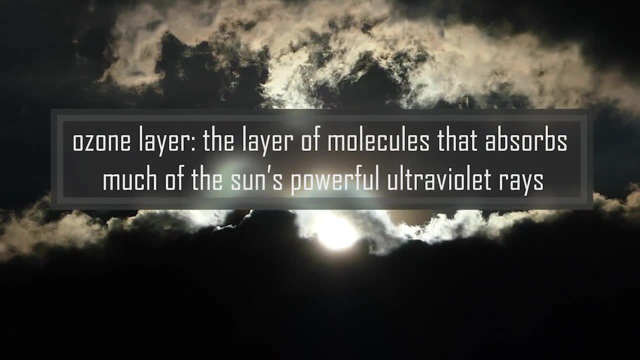 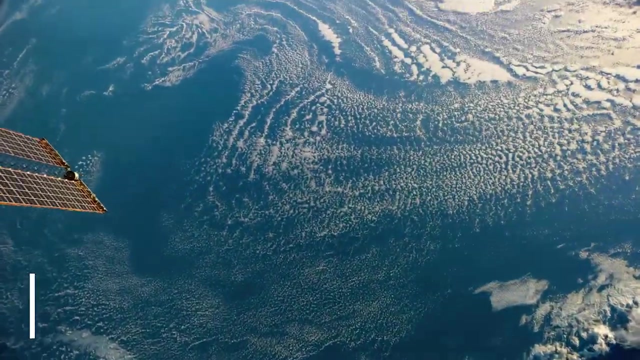 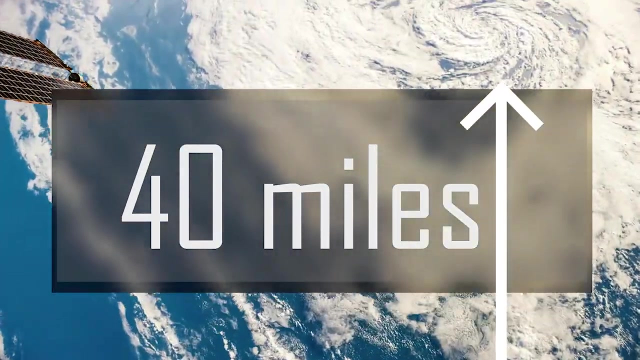 also contains the ozone. This layer of molecules absorbs much of the sun's powerful ultraviolet rays and protects life on Earth. All of these absorbed rays make the ozone layer quite warm. Just above the stratosphere is the mesosphere. This layer is about 40 miles above Earth's surface. Here meteors from space burn up. and are destroyed. Ironically, the mesosphere is the most important layer of the stratosphere. The mesosphere is the coldest layer of the atmosphere. The cold molecules scrape the incoming meteors, which cause friction and eventually fire. The mesosphere is so cold. 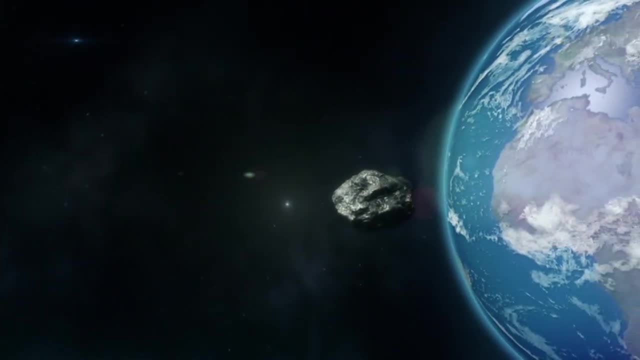 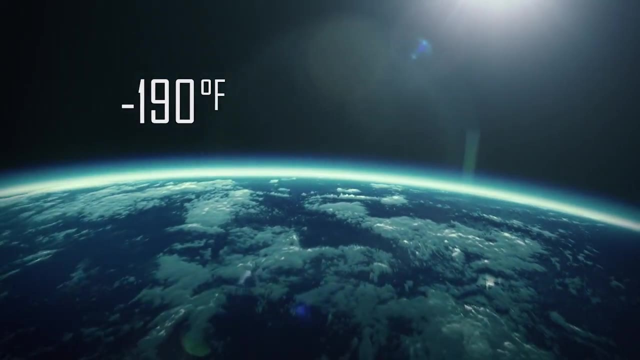 because it is far away from the absorbed heat of Earth, but still quite far from the sun. Temperatures can be as low as negative 190 degrees Fahrenheit. 300 miles up from Earth's surface is the thermosphere. The thermosphere is the coldest layer of the atmosphere. 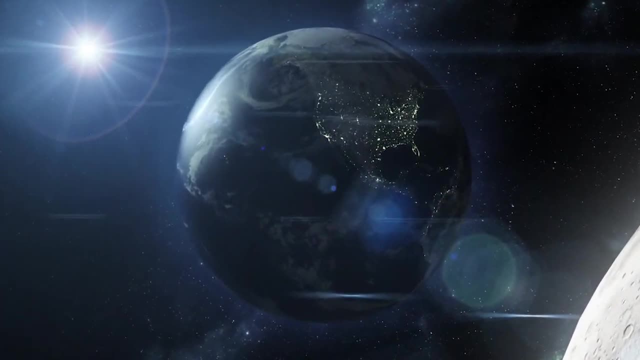 The mesosphere is the coldest layer of the atmosphere. The cold molecules scrape the incoming meteors, which cause friction and eventually fire. The mesosphere is the coldest layer of the atmosphere. This layer of the atmosphere is where space shuttles and satellites orbit the planet. 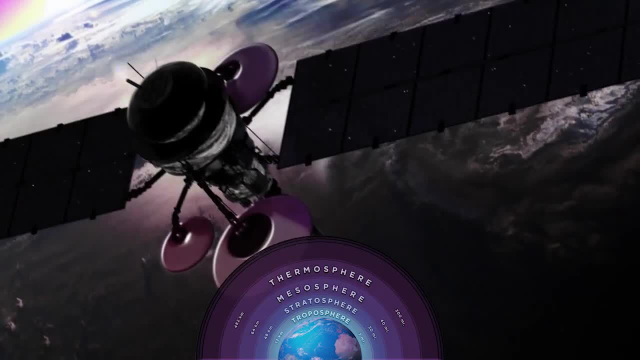 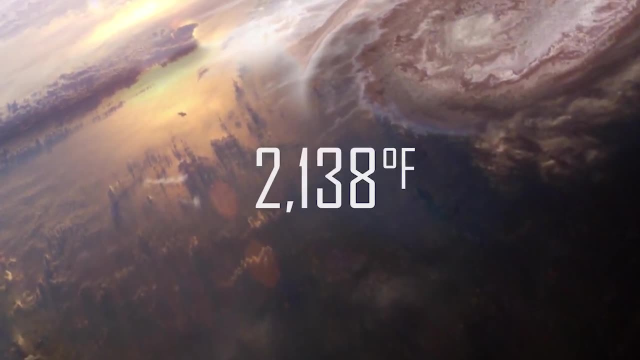 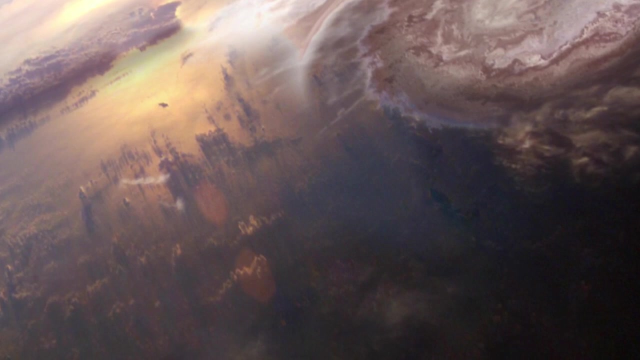 The temperature of the thermosphere is incredibly hot because of energy coming directly from the sun. At this level, temperatures can reach up to 2,700 degrees Fahrenheit. At this height, the air is quite thin and there are very few molecules. The final level of the atmosphere is called the 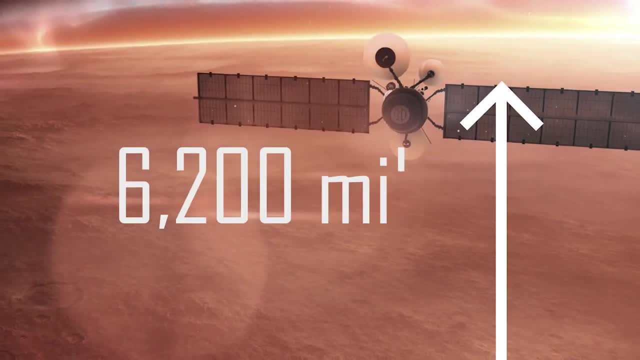 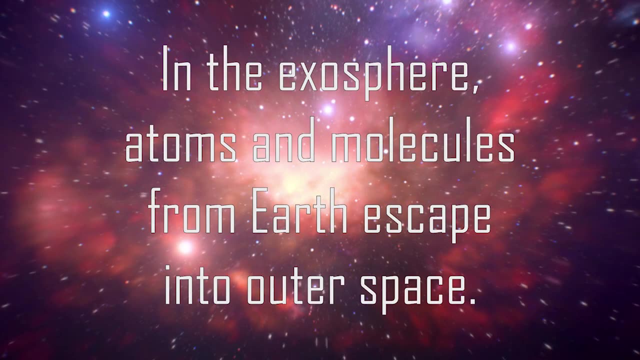 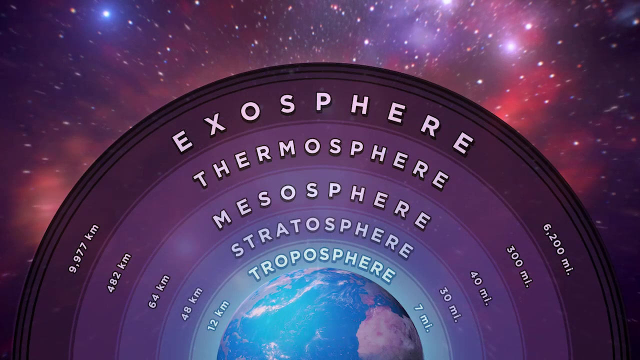 exosphere. It extends about 6,200 miles into space. In the exosphere, atoms and molecules from Earth escape into outer space and completely leave the planet's atmosphere. Temperatures can vary widely here, from very cold to very hot, depending on location. Although the five layers